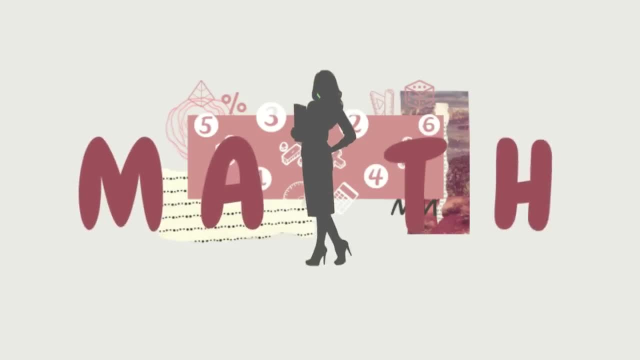 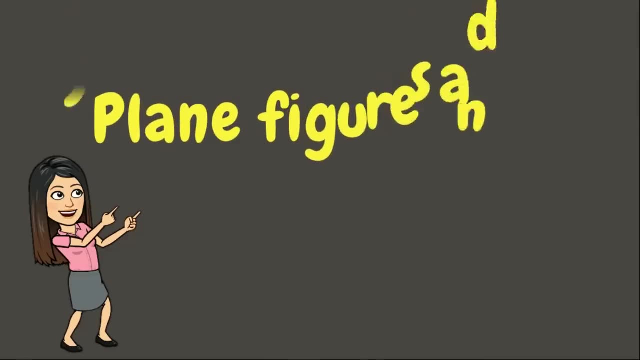 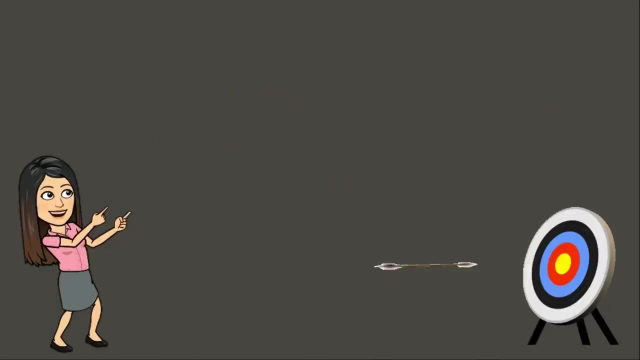 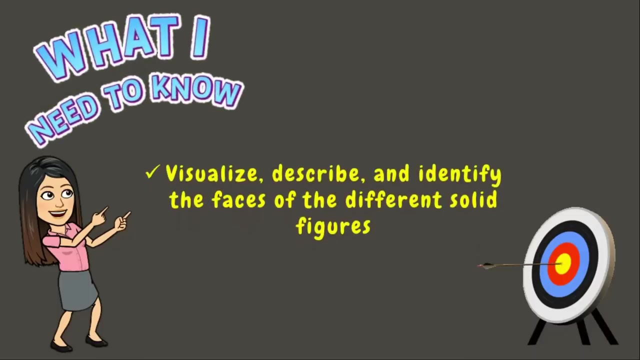 Plain Figures and Solid Figures. Good day students. Welcome back to my classroom For today's lesson. you are going to learn how to visualize, describe and identify the faces of the different solid figures and differentiate solid figures from plain figures. Let us begin. 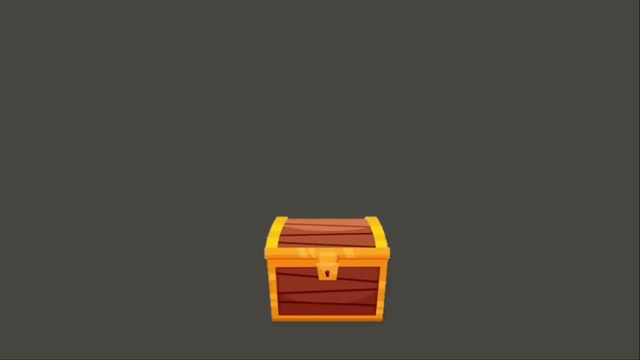 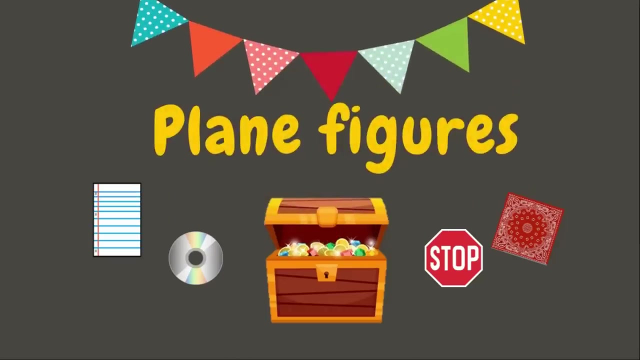 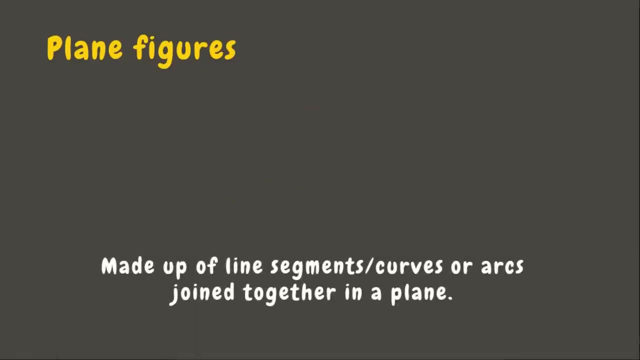 Let's go and have treasure hunt. Let's find out what's inside this treasure. We have stop sign, a piece of paper, handkerchief and a compact disc. These objects represent plain figures. Plain figures are made up of line, segments or curves or arcs joined together in a plane. 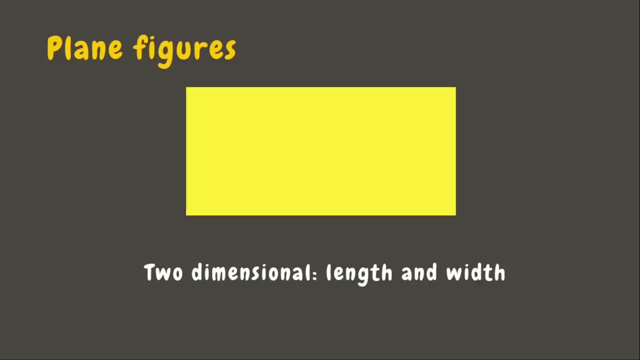 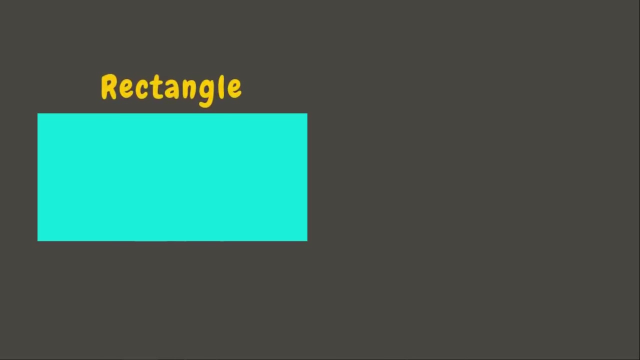 A plain figure has two dimensions, which are the length and the width, And, lastly, it has a flat surface that extends without end in all directions. Now let's learn some basic plain figures. The first one is a rectangle. A rectangle is a plain, closed figure enclosed by four line segments. 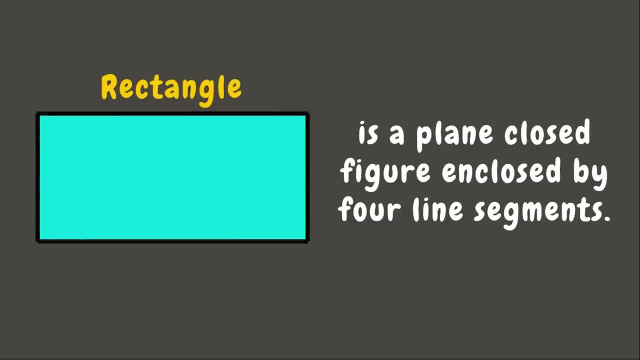 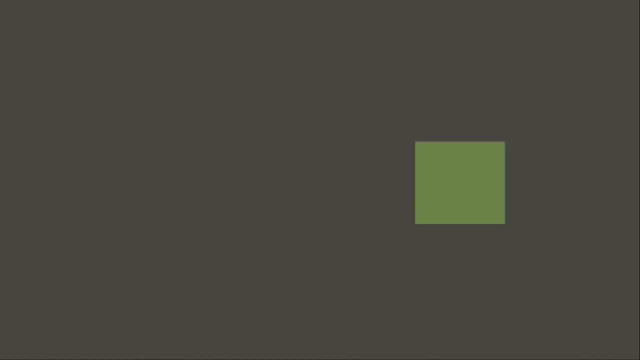 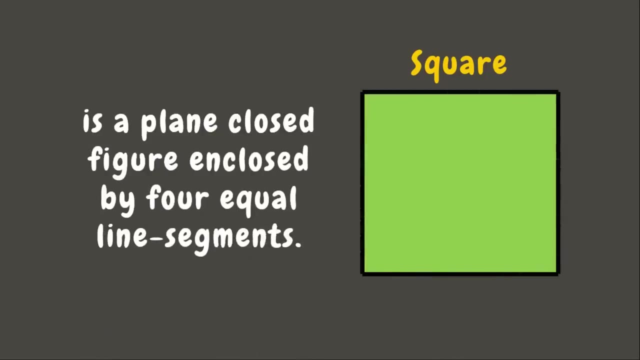 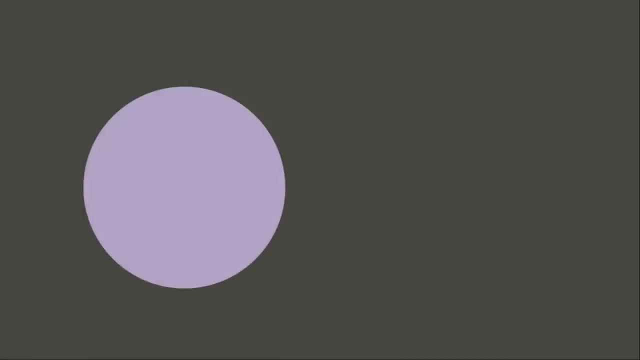 It has two pairs of equal sides: the lengths and the widths. Next one we have here: square A square is a plain, closed figure enclosed by four equal line segments. The next one we have: circle A circle is a plain, closed figure enclosed by a curve having no sides and no corners. 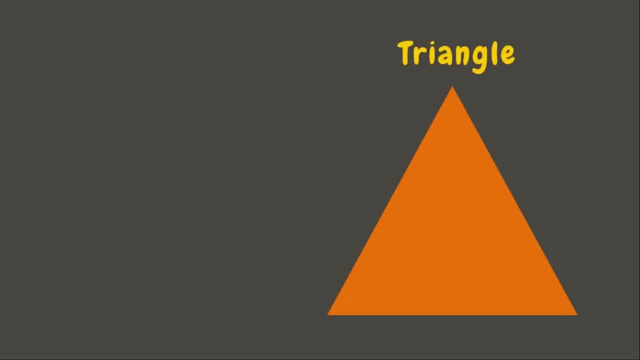 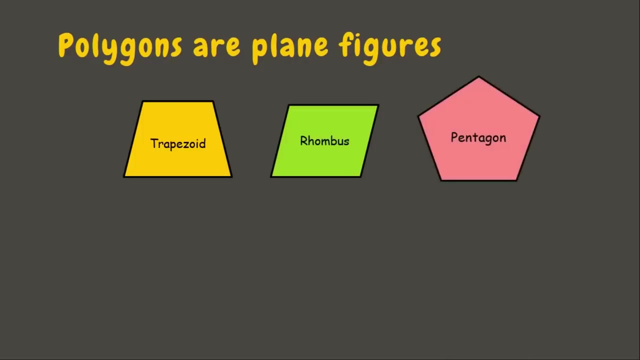 The next on the line is the triangle. The triangle is a plain, closed figure enclosed by three line segments. Now polygons are also considered as plain figures. Here are some examples: We have trapezoid, rhombus, pentagon. 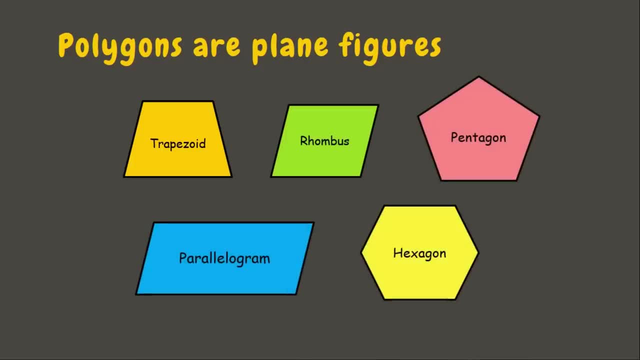 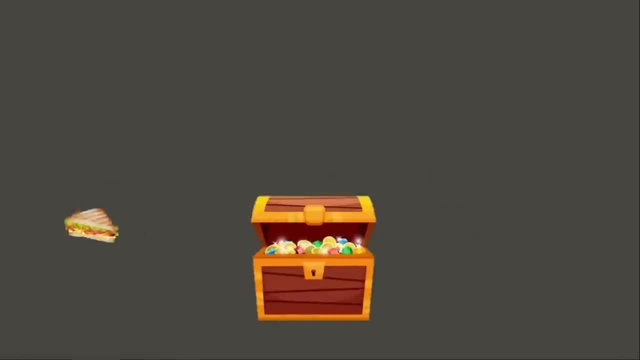 parallelogram, hexagon and many more. Now let's move on to our next treasure hunt. We have here a sandwich, a ball, a can of soda, a party hat, a bar of chocolate and a Rubik's cube. 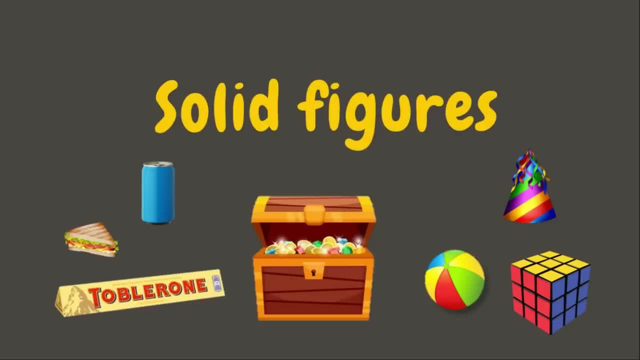 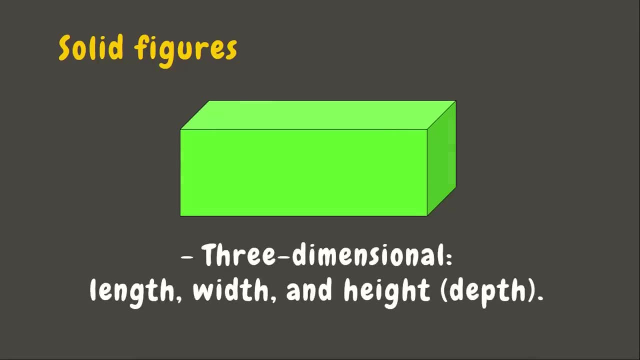 These are examples of solid figures. Solid figures has three dimensions. Solid figures has three dimensions. It has length, width and height. It has length, width and height. Now let's learn about the parts of the solid figure. Now let's learn about the parts of the solid figure. 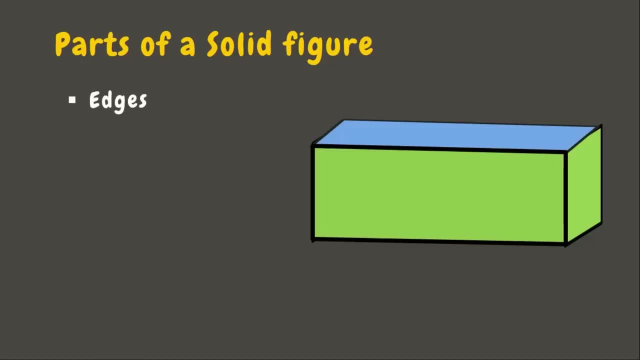 Now let's learn about the parts of the solid figure. First one is the edges. The edges are the line segments that meet or join together in order to create a figure. The edges are the line segments that meet or join together in order to create a figure. 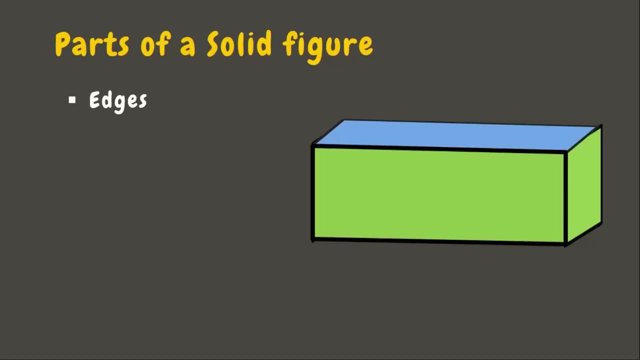 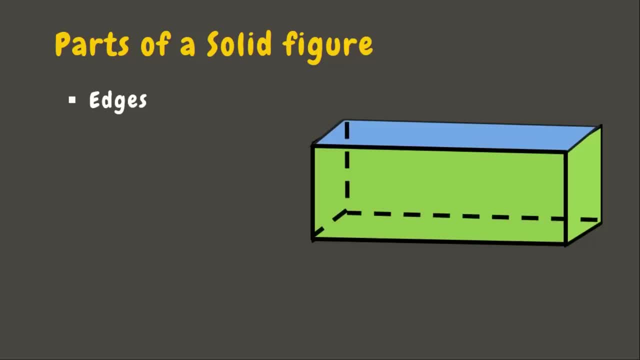 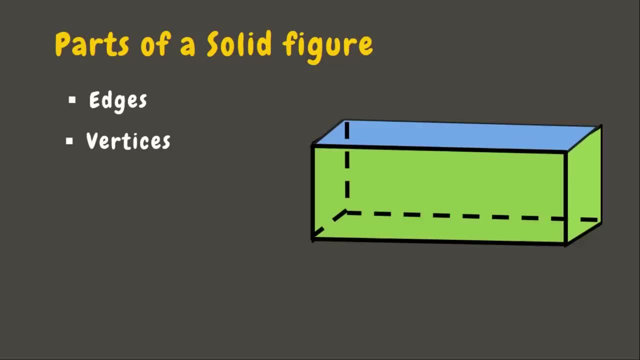 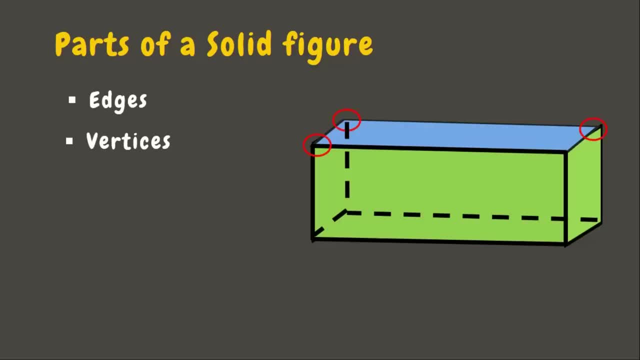 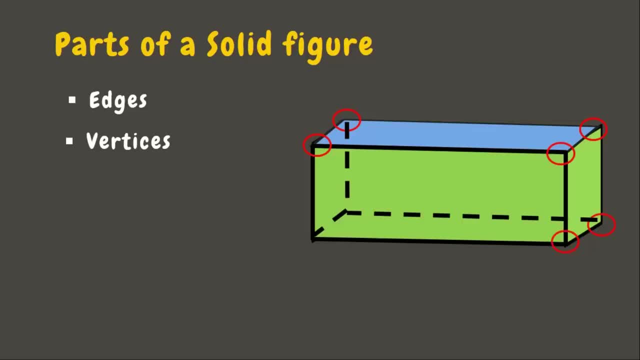 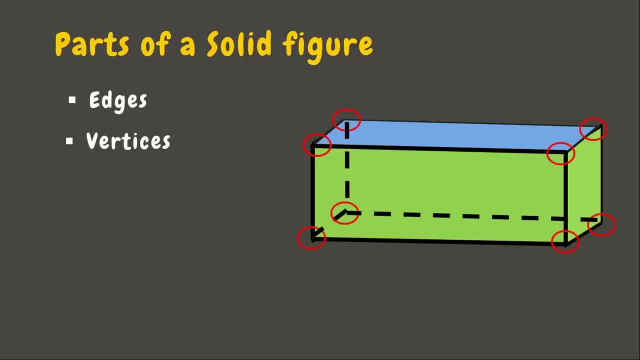 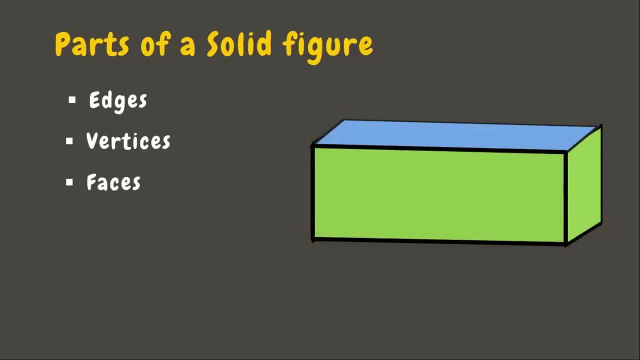 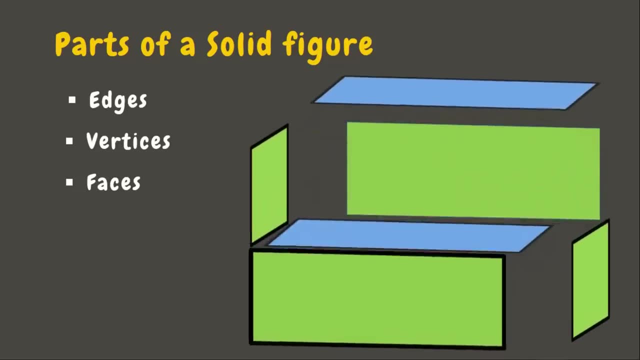 Next on the line is the faces. Next on the line is the faces. The faces are the flat surfaces of a figure. The faces are the flat surfaces of a figure. In the given figure, it has 6 faces. In the given figure, it has 6 faces. 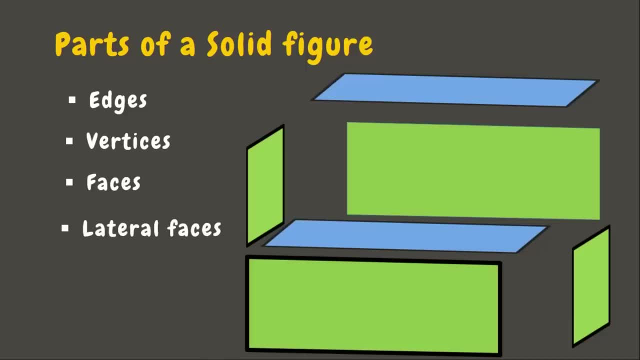 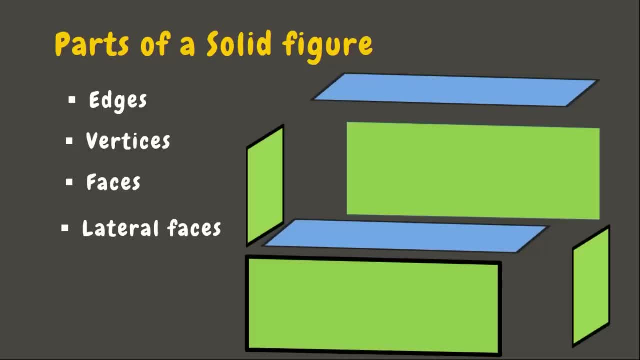 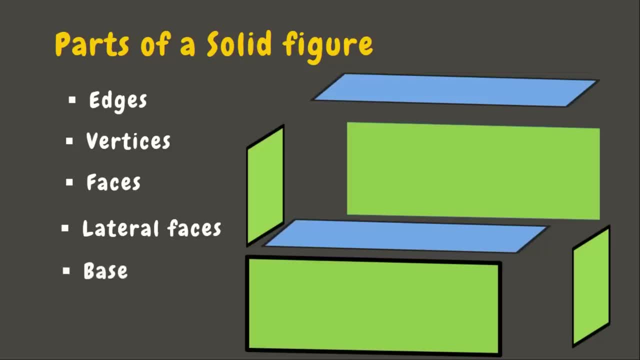 In the given figure. it has 4 lateral faces. Lastly, we have the base. The base is the top or the bottom part of the figure? The base is the top or the bottom part of the figure? This given figure has 2 bases. 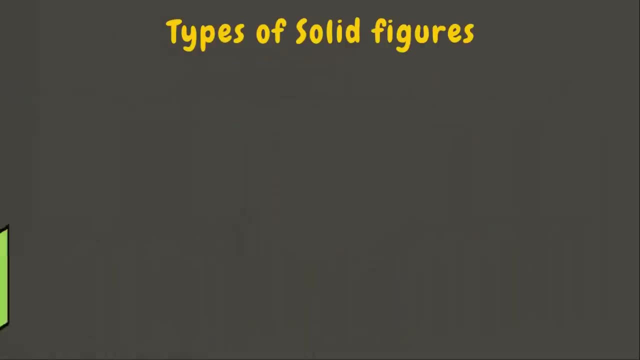 This given figure has 2 bases. This given figure has 2 bases. Now that you already know the parts of the solid figure, Now that you already know the parts of the solid figure, let's learn about the types of solid figure. Let's learn about the types of solid figure. 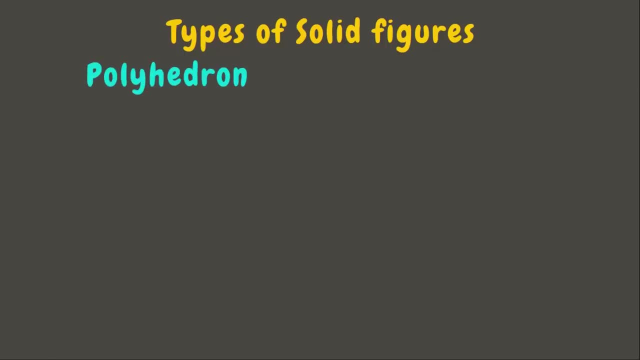 There are 2 types of solid figures. There are 2 types of solid figures: The polyhedron and non-polyhedron. The polyhedron and non-polyhedron: A polyhedron figure has flat surfaces. A polyhedron figure has flat surfaces. 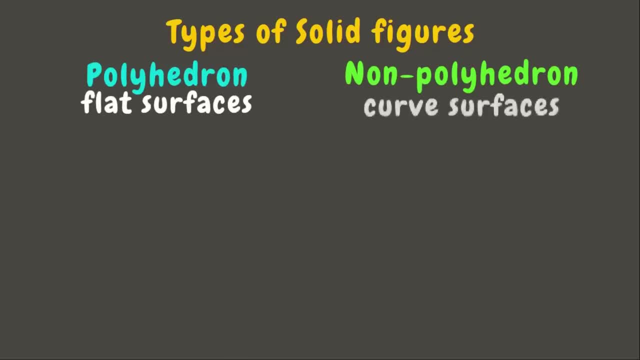 While the non-polyhedron figure has curved surfaces, While the non-polyhedron figure has curved surfaces, While the non-polyhedron figure has curved surfaces. Now, let's try and classify these objects. Now, let's try and classify these objects. 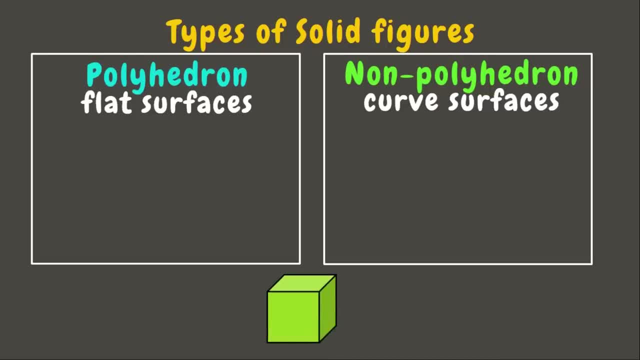 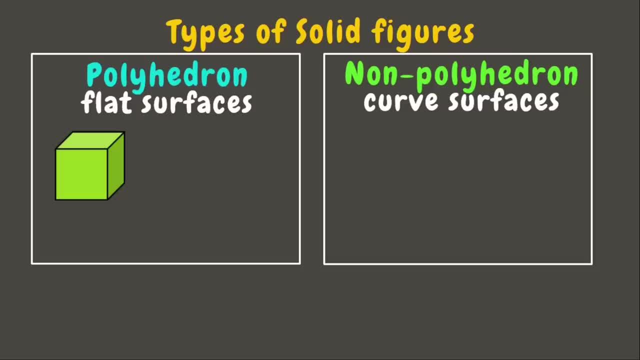 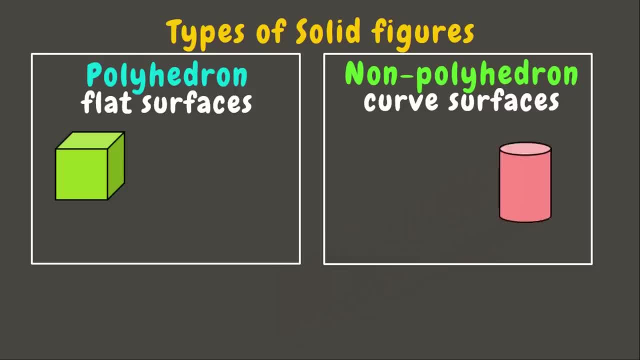 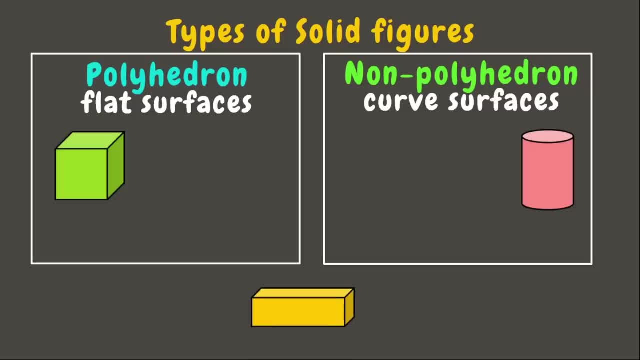 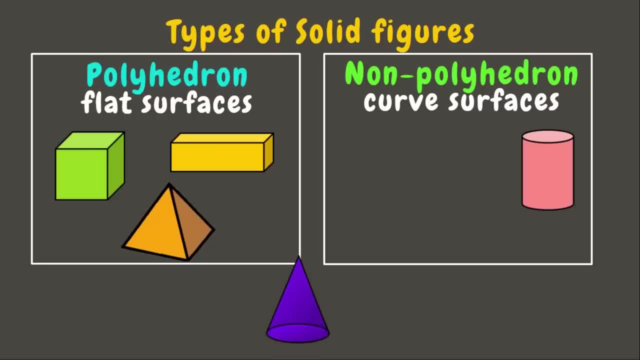 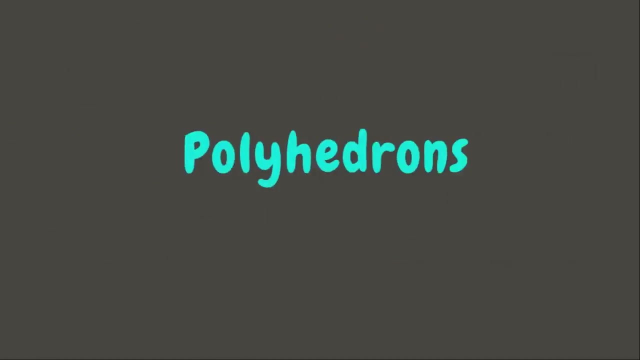 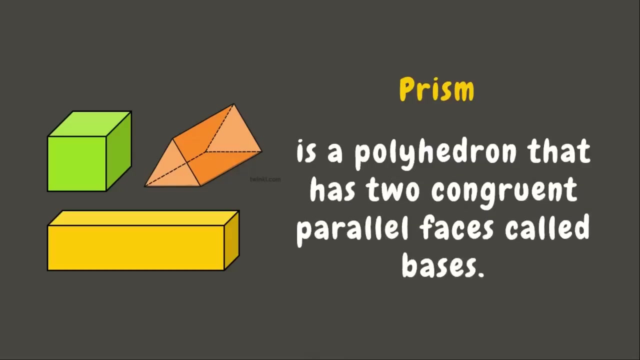 cone, and you are correct, it is a non polyhedron. and lastly, we have sphere: great job, it is a non polyhedron. wonderful, now let's learn more about polyhedrons again. polyhedrons are solid figures which have flat surfaces. first one: we have prism. prisms are polyhedrons. that has two congruent. 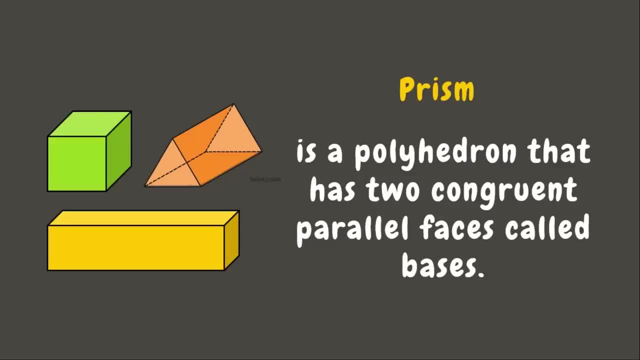 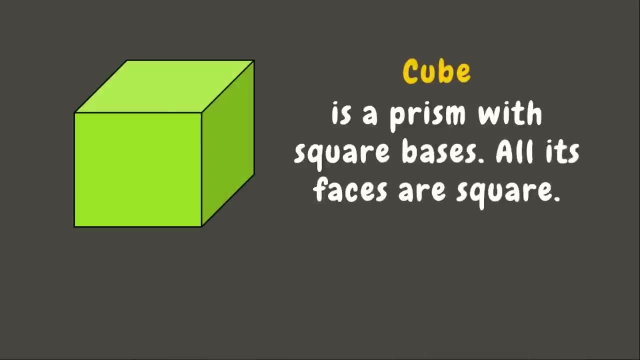 parallel bases called vases. so we have cuad, kali prism and iptangular prism and many more. let's talk about cube. a cube is a prism with square bases and all its bases are square. example of cube objects are a Rubik's Cube, ice cubes And a box. 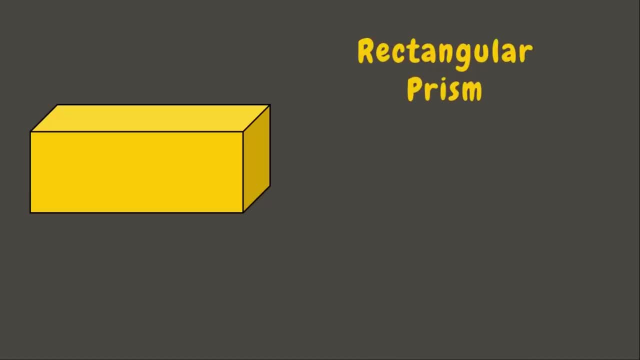 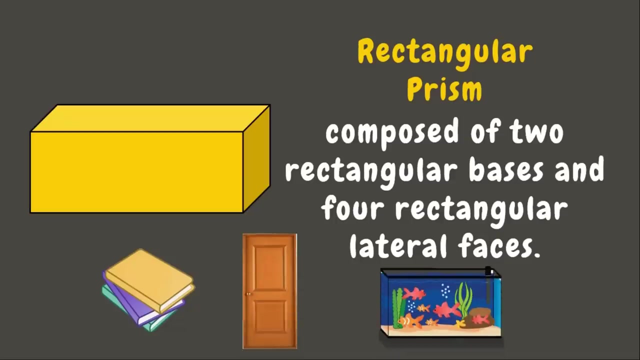 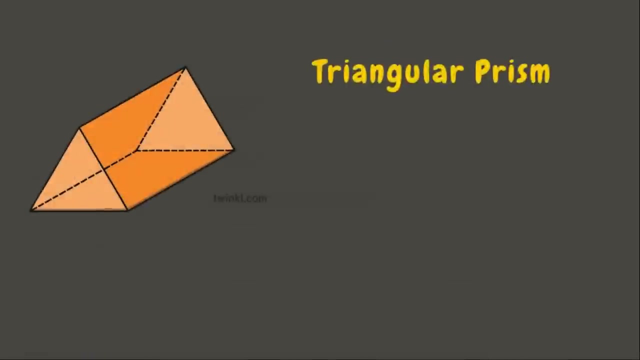 Next one: we have a rectangular prism. A rectangular prism is composed of two rectangular bases and four rectangular lateral faces. Examples of rectangular prism are a book door and an aquarium. Next in line, we have a triangular prism. Triangular prisms are composed of two triangular bases and three rectangular lateral faces. 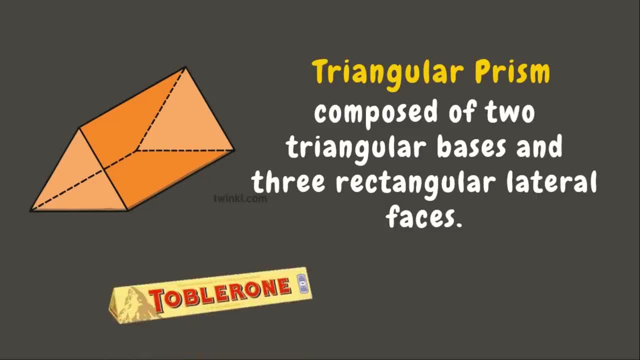 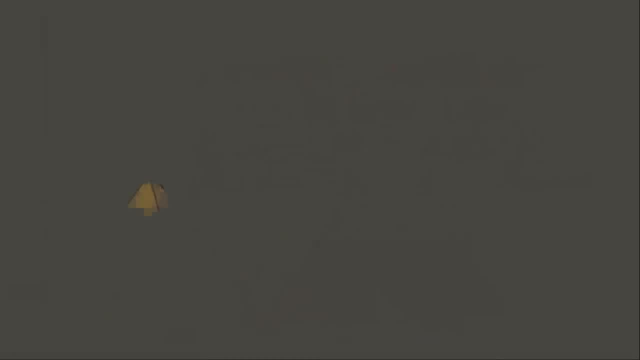 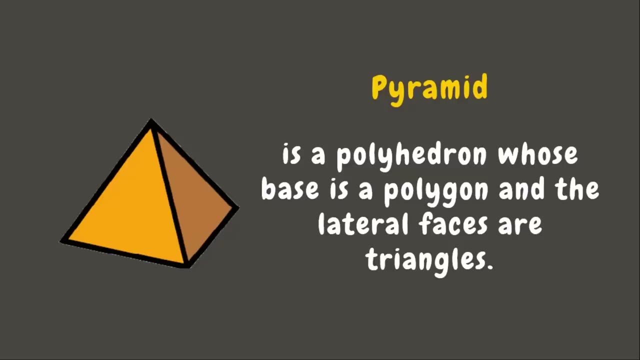 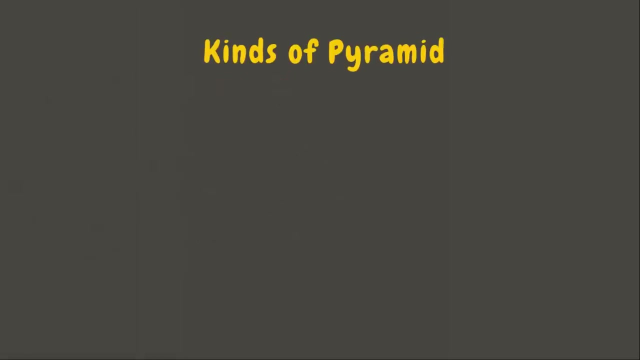 Examples of this are a chocolate bar, which have a triangular prism figure and a tent. Next one: we have a pyramid. A pyramid is a polyhedron whose base is a polygon and the lateral faces are triangles. There are different kinds of pyramid. 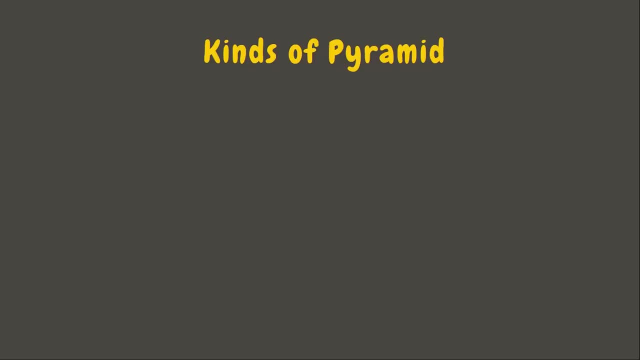 A pyramid is named after the shape of the base. Let's take a look at some examples. Since this pyramid has a triangular base, this is called triangular pyramid. Next one is: This is a pyramid which has a square as the base, And this is called square pyramid.